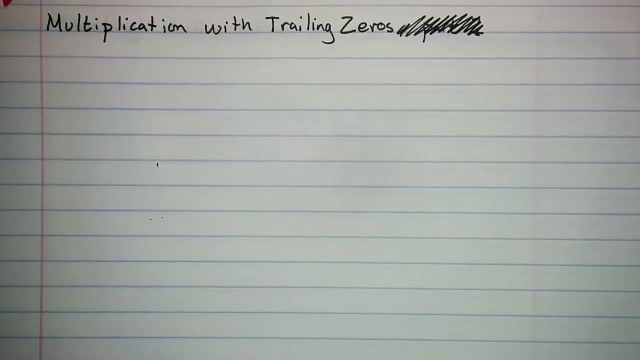 Earlier we talked about what happens in multiplication when we have a single digit followed by a bunch of zeros, So only one non-zero digit. A lot of the simplification that that gives. the multiplication process continues to stick around when we have several digits followed by trailing zeros. 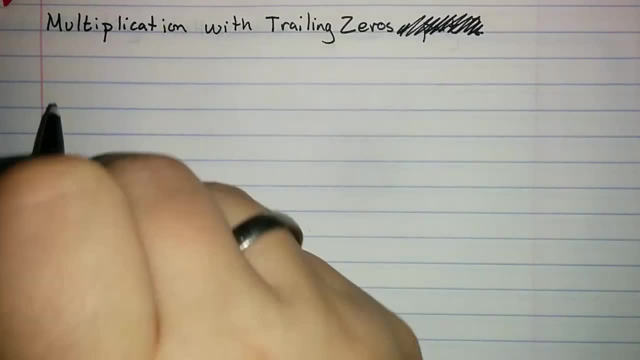 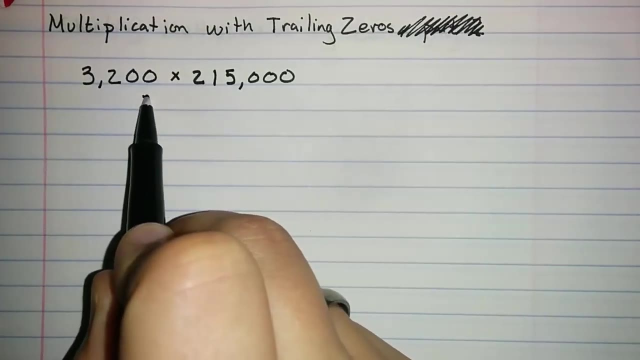 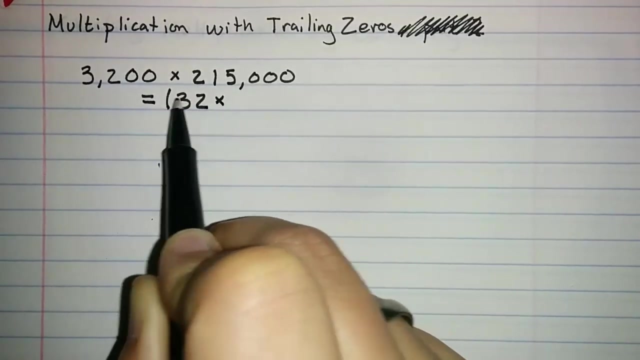 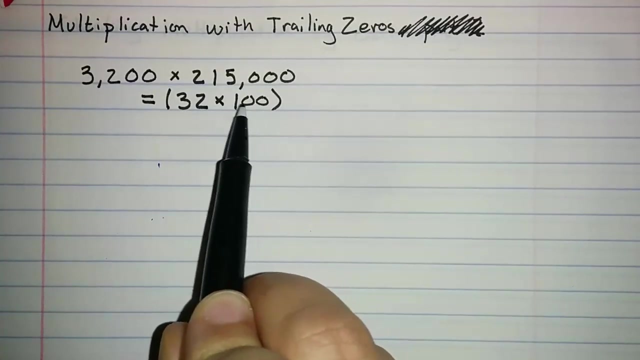 So, for example, let's say we want to multiply 3,200 times 215,000.. Well, remember 3,200, that's just 32 hundreds, Right? 32 with two zeros at the end is what we get when we multiply 32 by 100.. 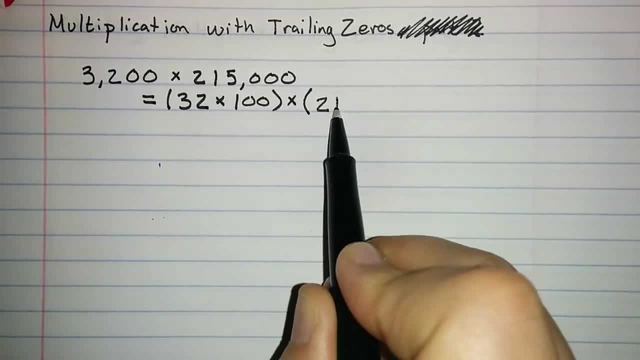 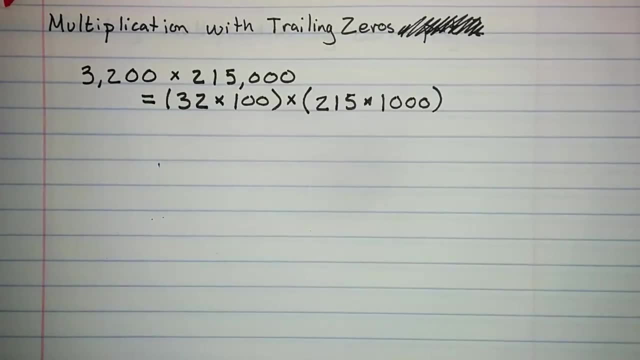 215,000.. That's just 215 groups of 1,000 each. So, again using the associative and commutative properties, we say that this is the same as 32 times 215 times 100 times 1,000.. 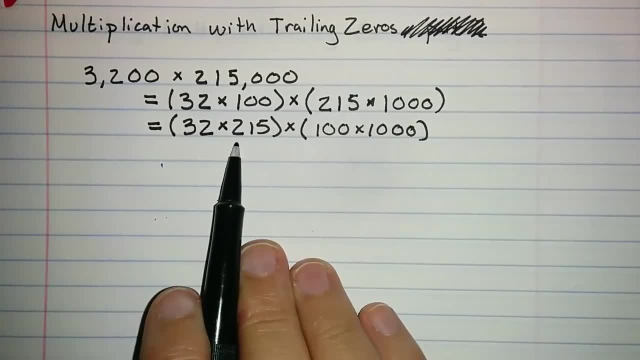 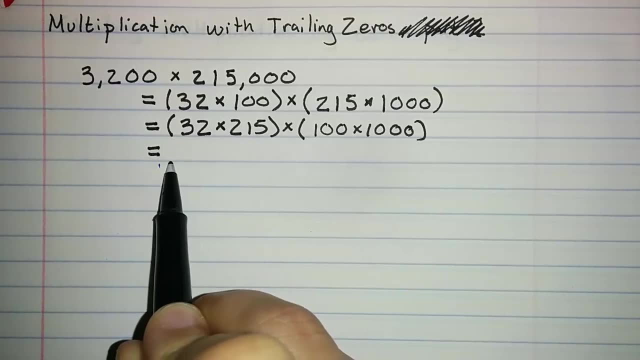 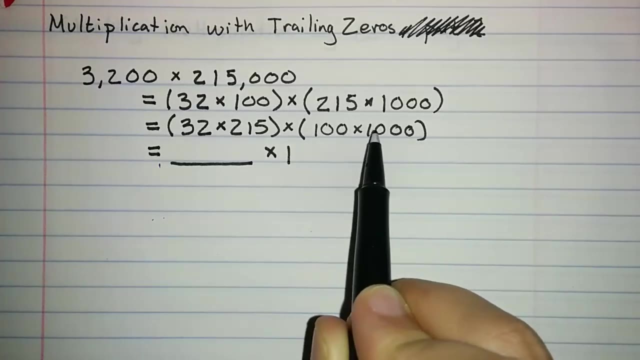 Now, when these were one-digit numbers, this step was easy. These are now multi-digit numbers and this step is a little bit easier. It's a little bit complicated, But it's going to be something, And that'll be multiplied by 1, followed by 1,, 2, 3, 4, 5 zeros. 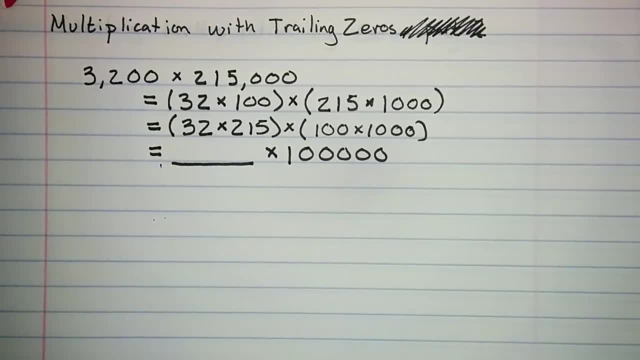 Let's work out what 32 times 215 is. Now I could write this as 32 times 215.. But did you notice how the standard algorithm for multiplication gets longer and longer the more digits we have in the second factor, Through the magic of the commutative property? 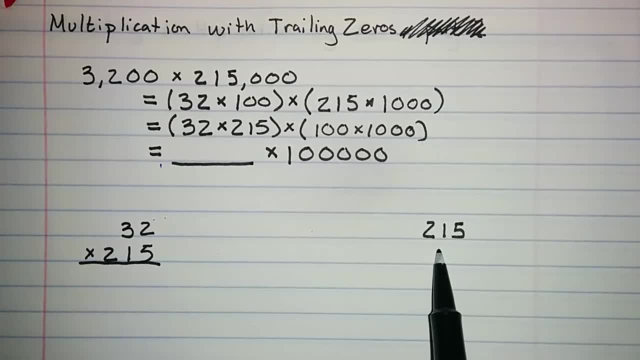 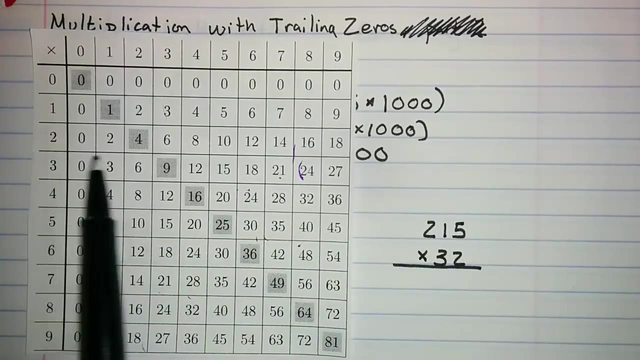 I can also write this in this order. But written in this order, the actual computation gets a little bit easier because I only have to deal with two digits. So let's do it: 2 times 5 is 10.. Carry the 1, write down the 0.. 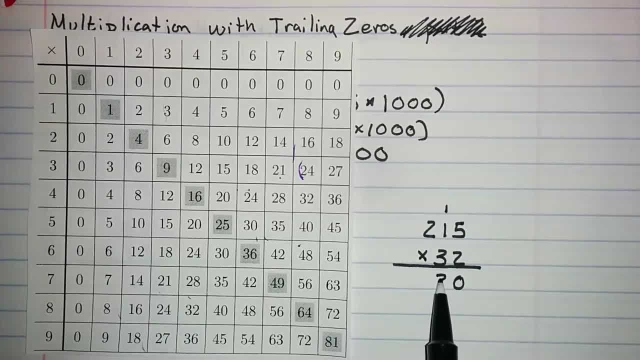 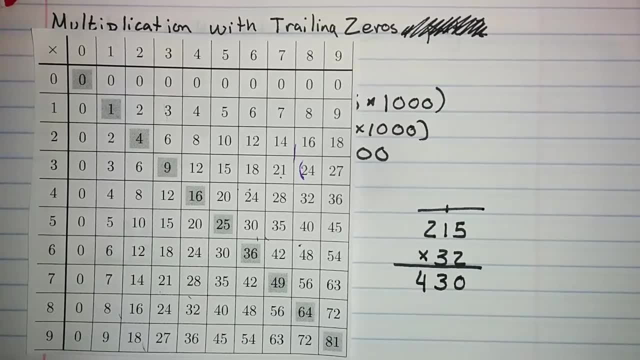 2 times 1 is 2.. Add in the 1, and I get 3.. 2 times 2 is 4.. Now cross off the old carries And my first digit is going to go in the tens place. 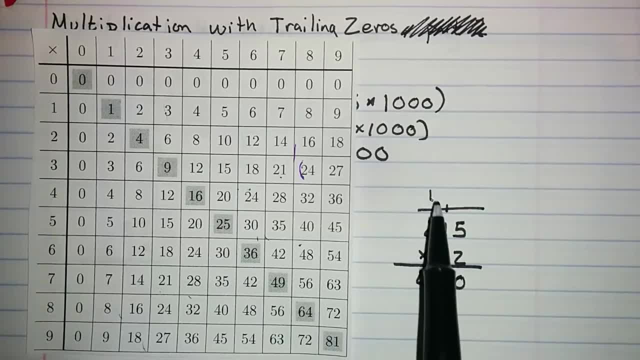 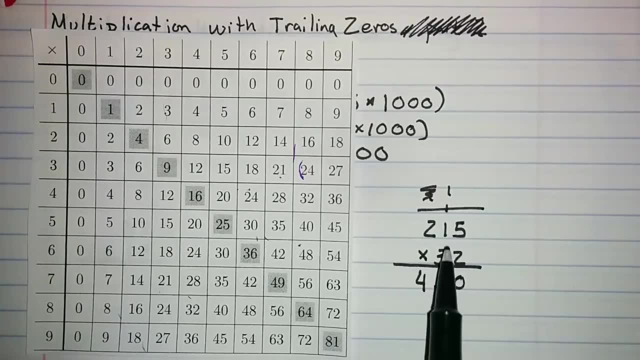 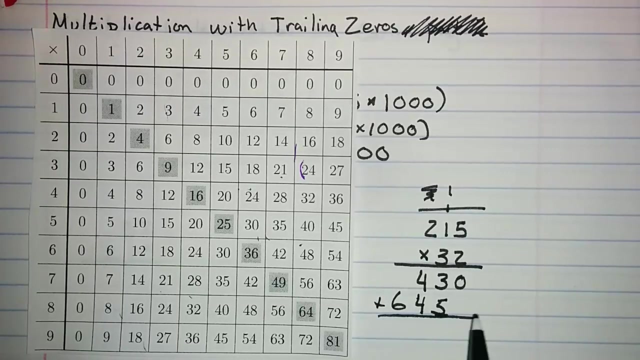 3 times 5 is 15.. Carry the 1, write down the 5.. 3 times 1 is 3,, plus another 1 is 4.. 3 times 2 is 6.. Now I'm ready to add. 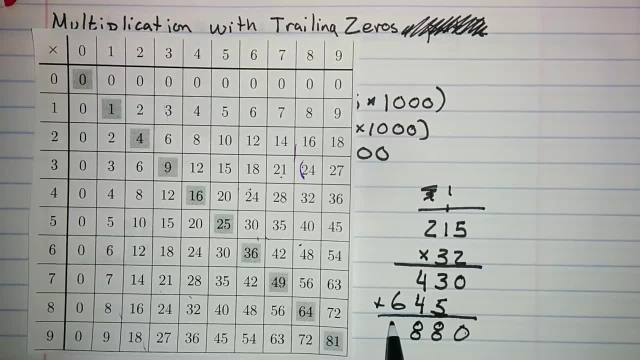 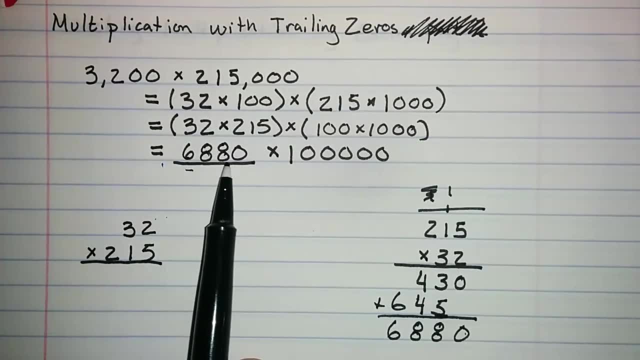 0, 8,, 8, 6.. So 32 times 215 is 6,880.. 100 times 1,000 is 100,000.. This big product is 6,880, and then 5 more zeros. 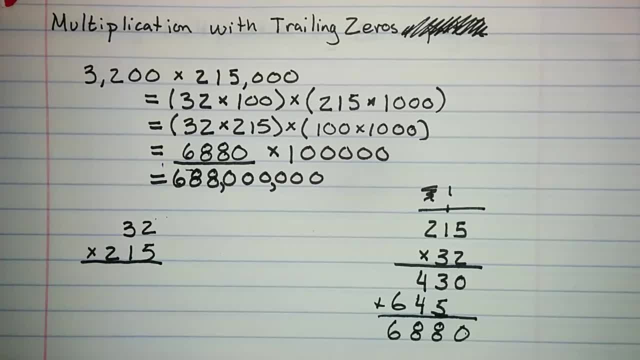 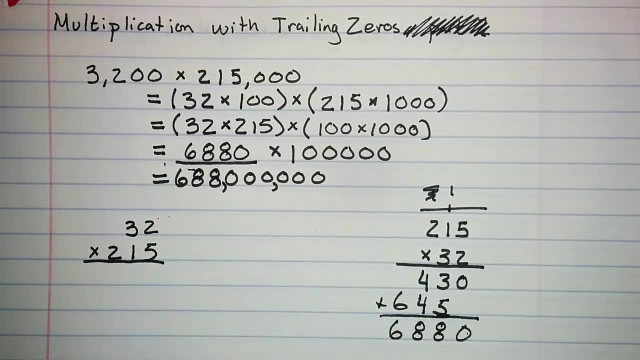 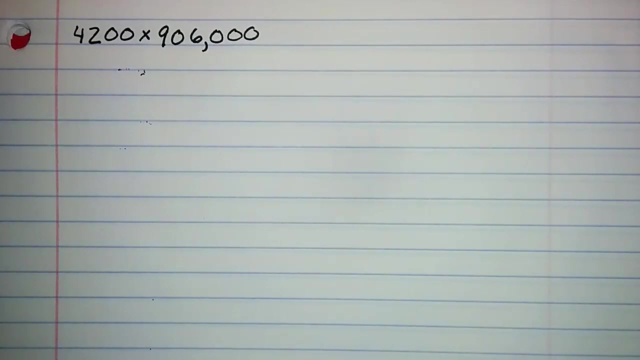 So 688 million Now. this is a perfectly okay way to work this problem, but it's an awkward way to write it. Let me show you a less awkward way to write a problem with trailing zeros. Let's say we want to multiply 4,200 times 906,000.. 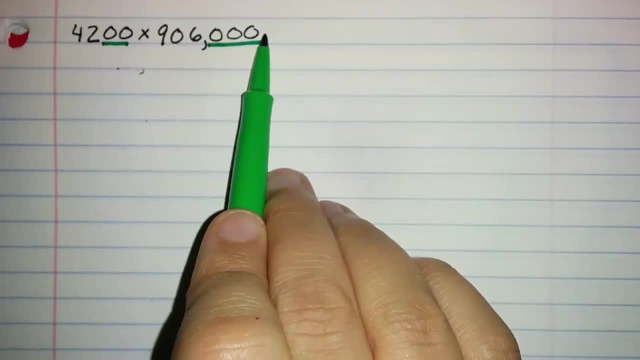 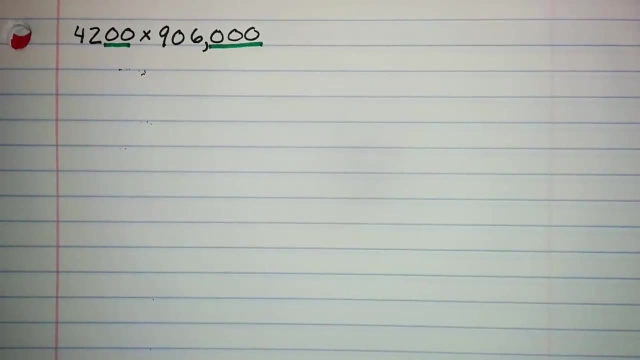 The first thing I want you to note: these are the trailing zeros in this number. these are the trailing zeros in this number, The zero between the 9 and the 6, we're going to really have to deal with that. We can't just pull it off the end. 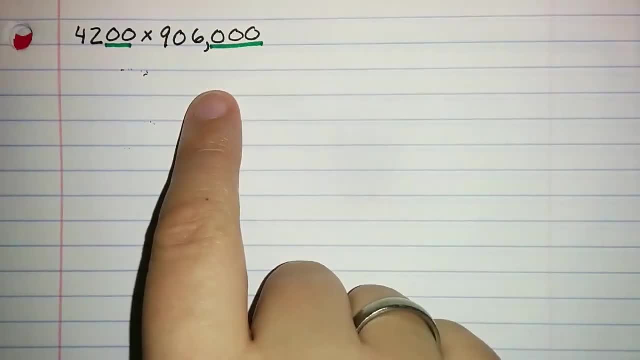 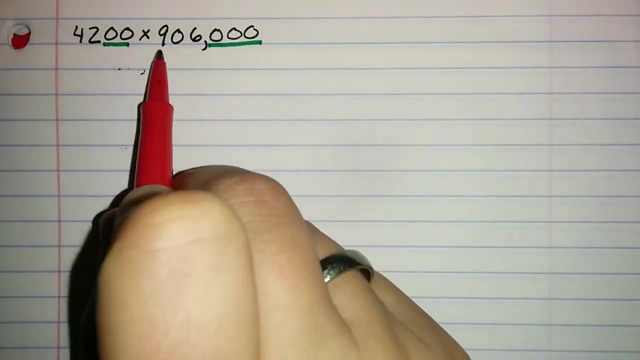 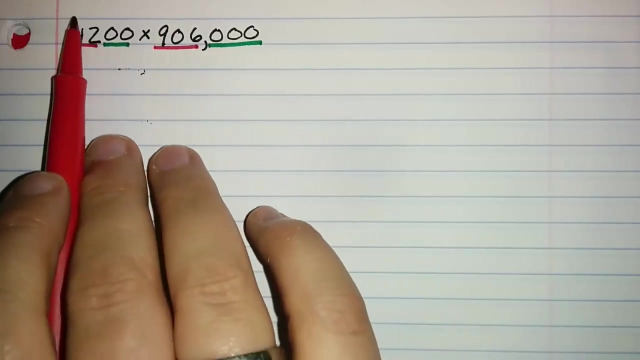 Because this is 906 times 1,000.. It's not anything times 10,000.. Looking at how many digits before the trailing zeros we have, I see this one has 3 digits before the trailing zeros. this one only has 2.. 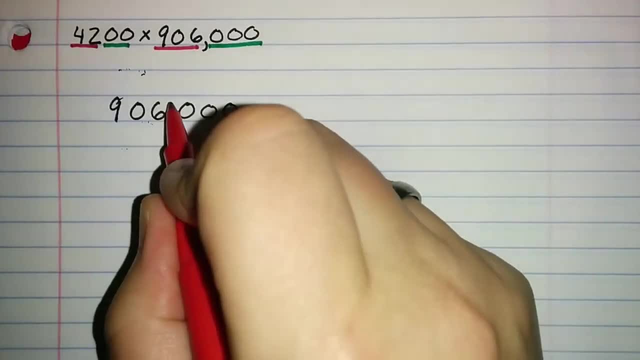 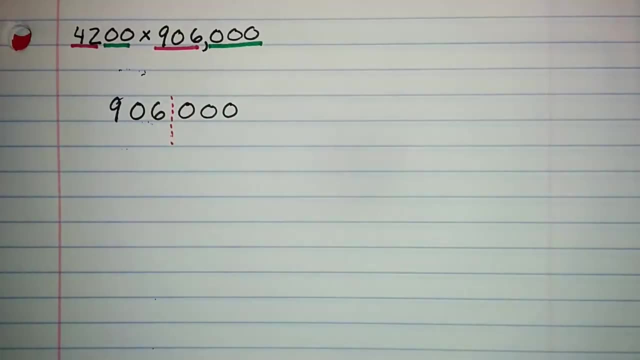 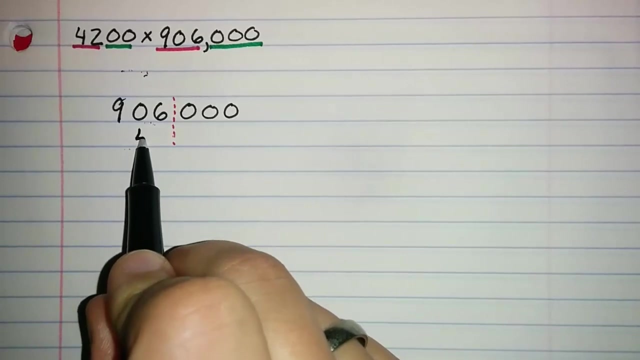 I'm going to write this number on top and I'm going to make a little dotted line between the digits I actually have to work with And the trailing zeros I'm just going to tack on at the end. This number has 2 digits before the trailing zeros. 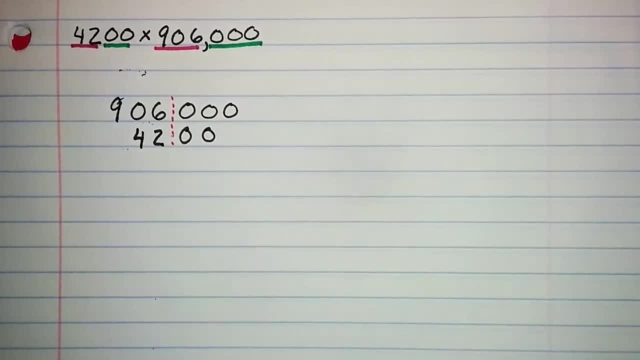 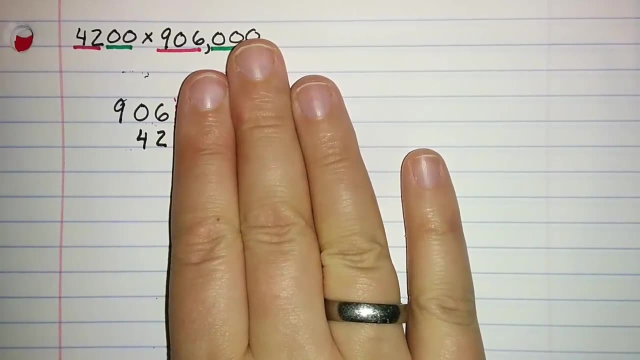 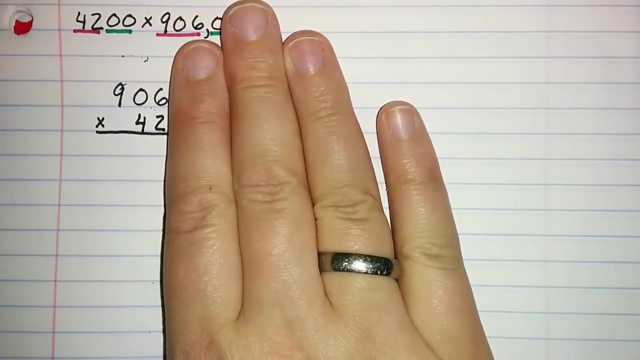 and then 2 zeros at the end. Notice, I did not line up the ones place, I just lined up the places I'm going to work with. It's as if I were setting up this problem, So now I'm going to ignore the trailing zeros for the moment. 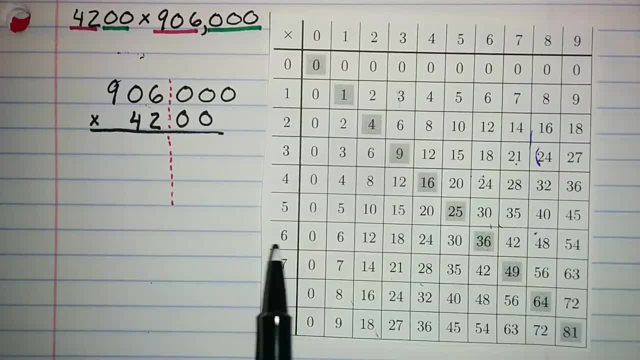 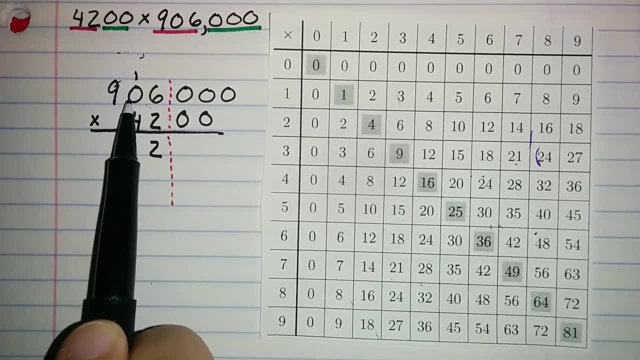 I'm going to continue that work. I'm going to do the red line. I'm going to multiply 2 times 6 is 12.. Carry the 1 right down the 2.. 2 times 0 is 0, plus 1 is 1.. 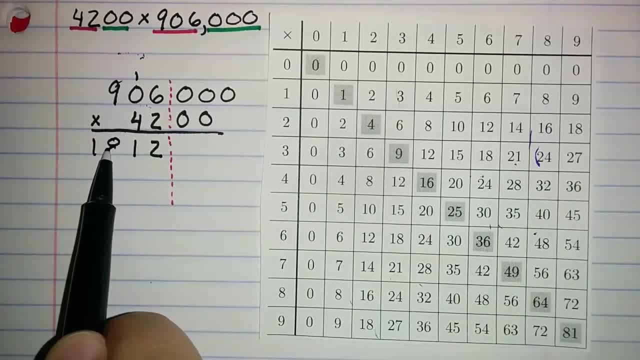 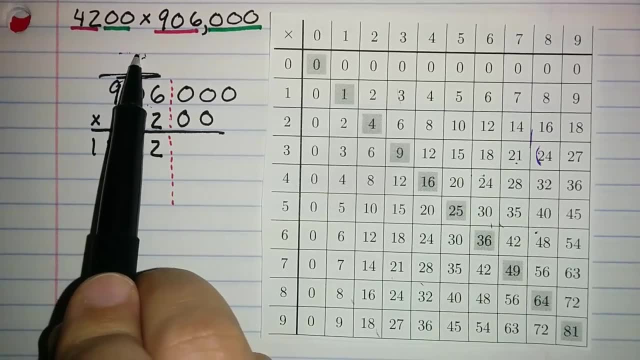 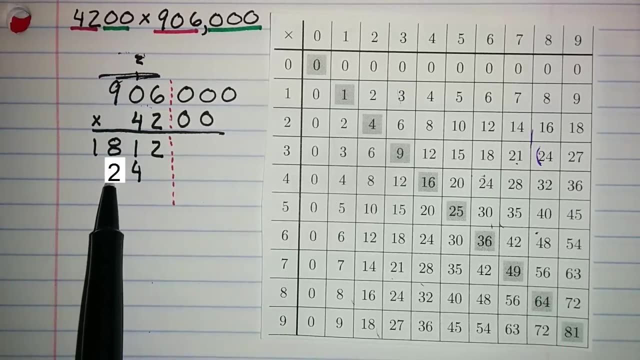 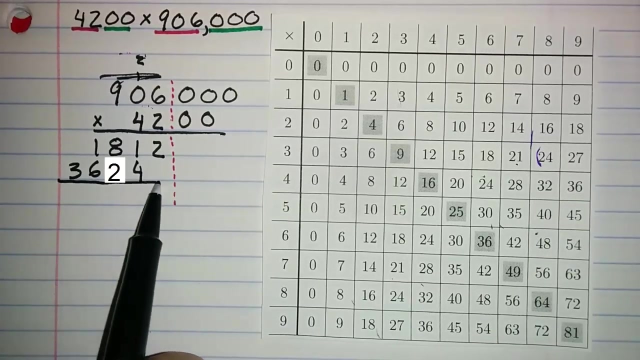 2 times 9 is 18.. Cross off the old carries: 4 times 6 is 24.. 4 times 0 is 0.. 4 times 9 is 36.. Now I'm going to add up, still ignoring the trailing zeros. 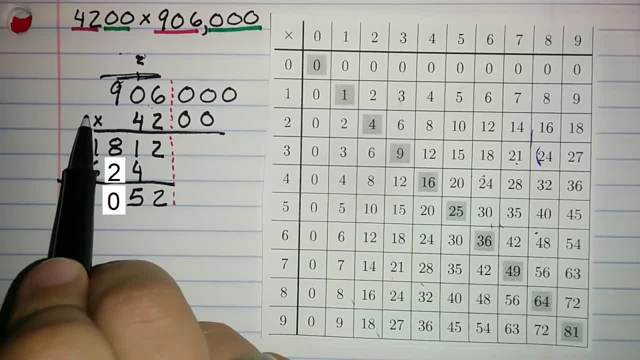 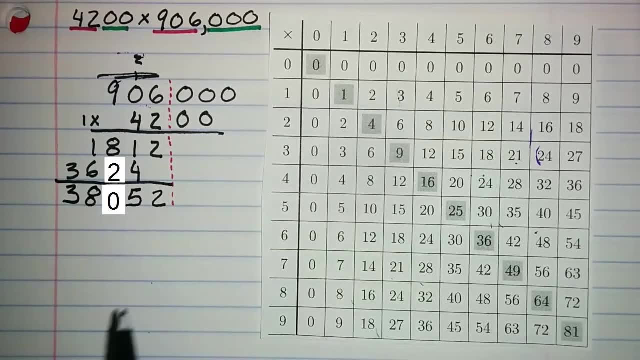 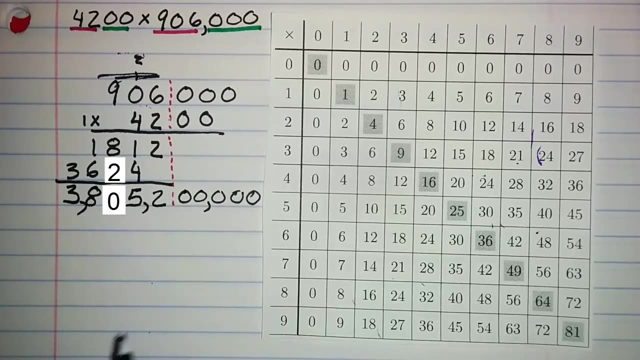 2,, 5,, 2,, 8,, 3.. Now, at the very end, I have 1,, 2,, 3,, 4,, 5, zeros on the end. Ooh, units, thousands, millions, billions. 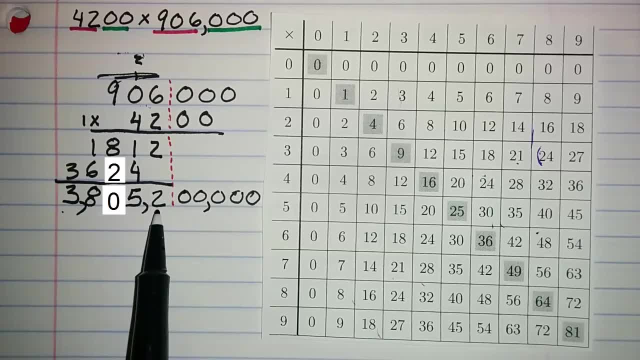 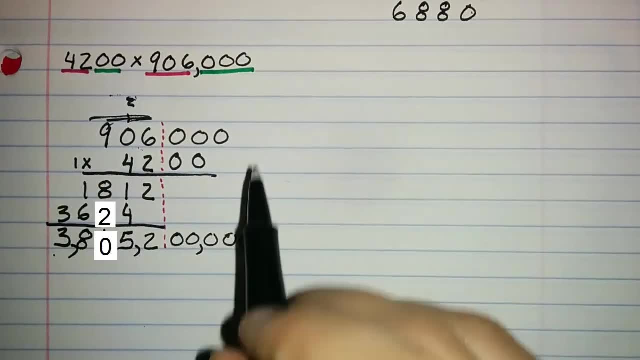 My product is 3,805,200,000.. Big numbers, But we didn't have to work that hard because we set aside the trailing zeros. I'm going to have you try one of these Again. I'm going to ask you to try this using this technique. 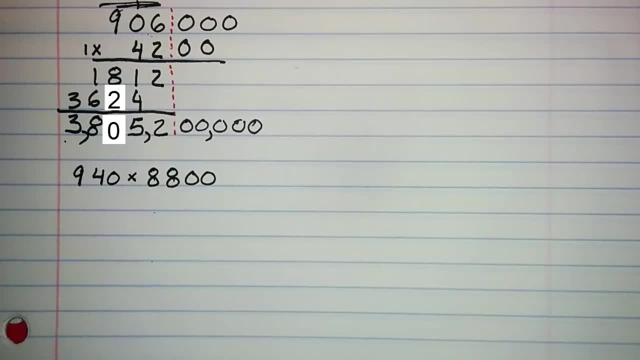 940 times 8,800.. Pause the video and try this now. Okay, So I'm going to have 940.. Noticing that each of these numbers has 2 digits before the trailing zeros, so the order doesn't really matter. 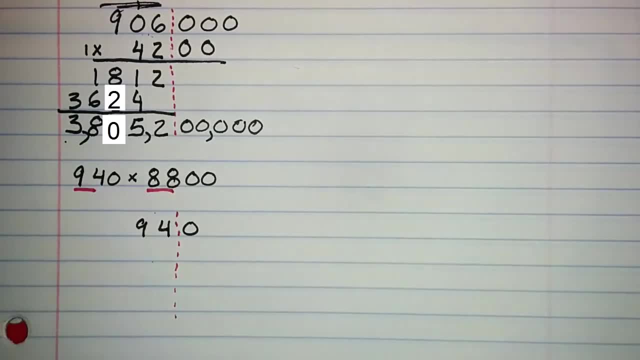 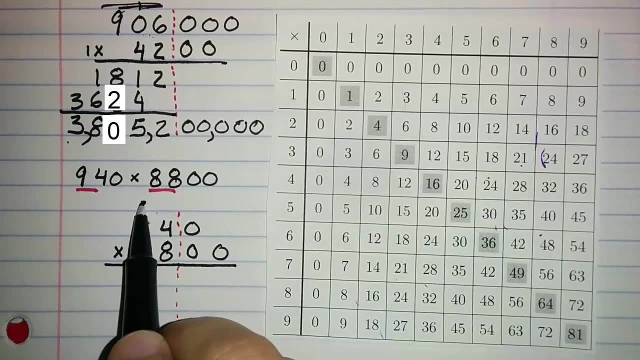 I'm going to put this dashed line walling off the trailing zeros. Here I'll have 88, followed by 2 zeros. 8 times 4 is 32.. 8 times 9 is 72, plus the 3 I carried is 75.. 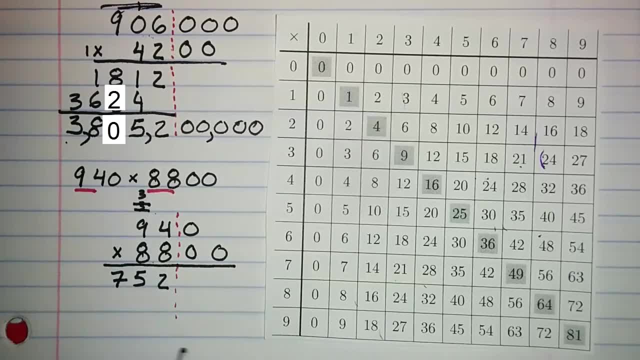 8 times 4 is 32.. Writing down the 2 now in the tens place because I'm multiplying by the 8 in the tens place: 8 times 9 is 72, plus the 3 I carried is 75.. 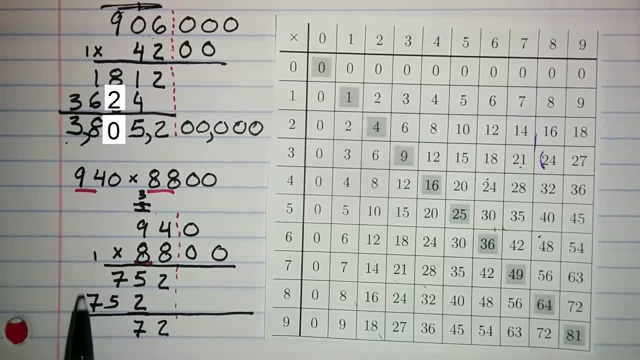 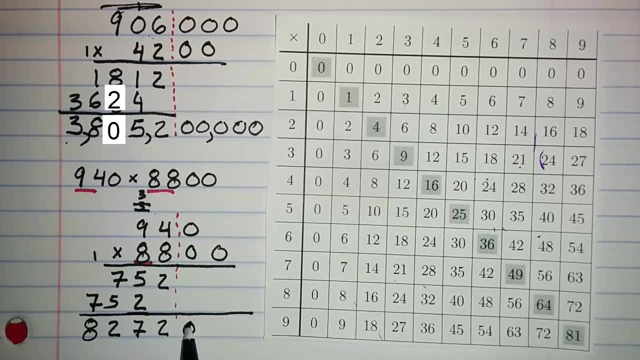 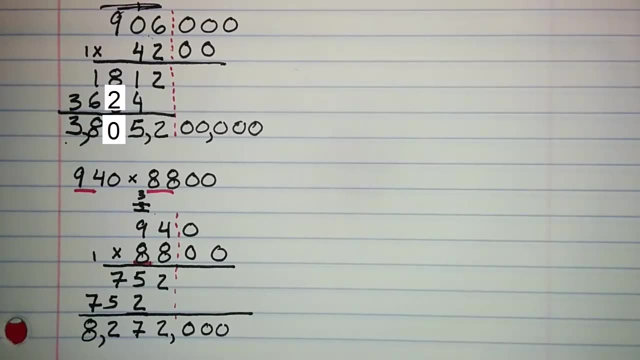 So what do I have? 2,, 7,, 12,, 8.. And then 1,, 2,, 3 trailing zeros, 3 trailing zeros, 1,, 2,, 3 trailing zeros. My answer is 8,272,000. 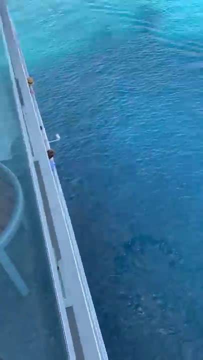 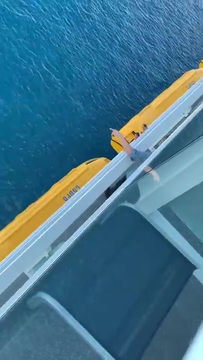 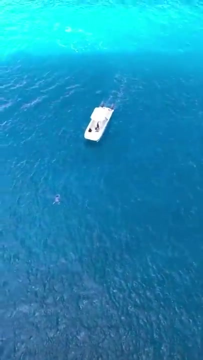 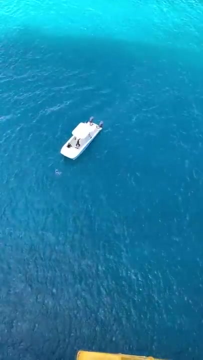 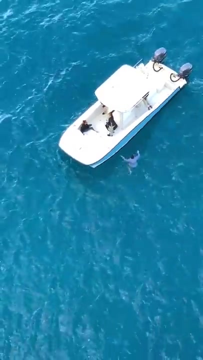 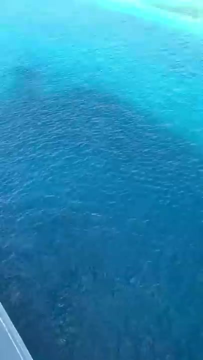 This video was made possible by the support of the US Department of Education and the US Department of Education and the US Department of Education. This is an educational video. Please add punctuation in the appropriate places.